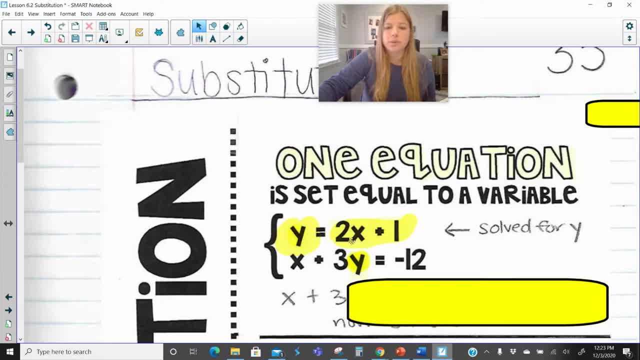 it's going to be now 3 times every, So I'm going to take everything y is equal to. I'm substituting 2x plus 1 in for y And I need to put parentheses around that entire expression and then bring down equals negative 12.. 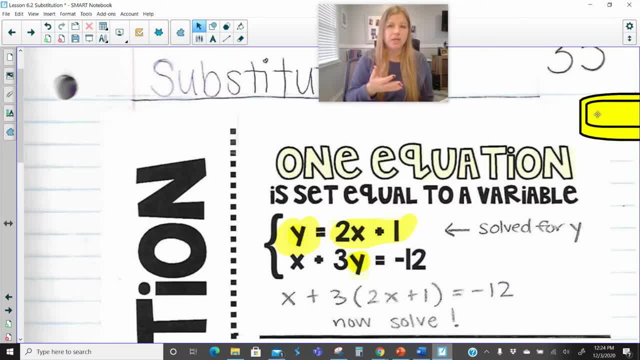 Now remember, substitution means that you're replacing something with something of equal value, Like if you were to go to the diner and you said: I would like to substitute my french fries for a baked potato, Or I would like to substitute my french fries for onion rings. 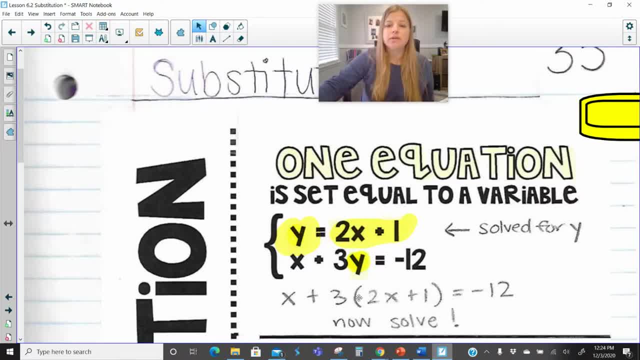 They would swap that out, You wouldn't get both. So notice here: y in this new equation. And after you get this equation, you then go ahead and you're able to solve for x, Because, notice, you don't have two different variables now in this equation. 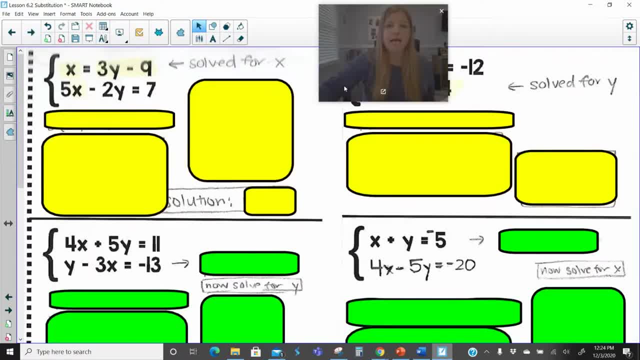 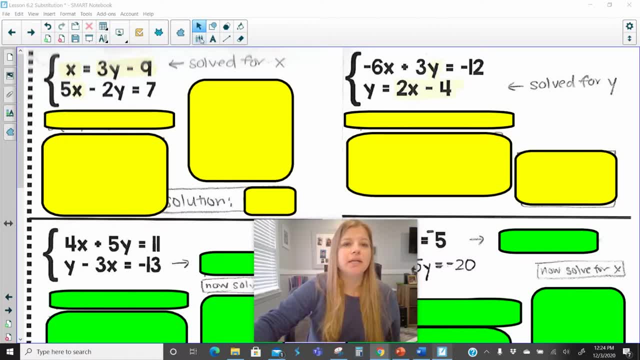 You only have one, So let's take a look at a couple of problems of this particular type, And they're going to be both up here in yellow, So let's take a look. This first equation: x equals 3y minus 9.. 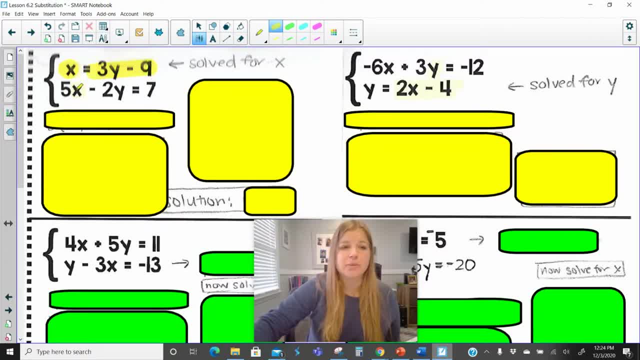 That means everywhere we see x in the other equation, in this one spot here we're going to substitute, And we're going to substitute in everything that x is equal to. So this second equation now becomes 5- in parenthesis, 3y minus 9.. 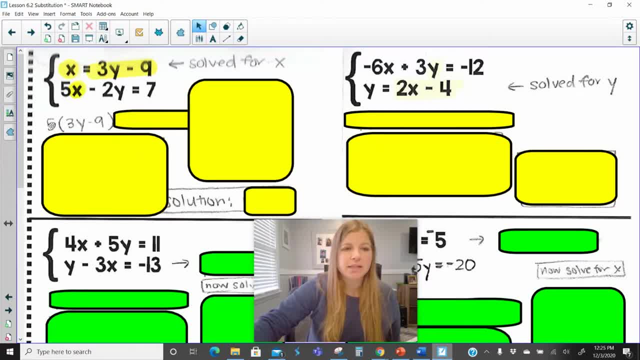 Close my parenthesis And so, notice, that's my 5x here And now I'm going to just continue to bring down the rest of the equation. Minus 2y equals 7.. Notice, I only have the variable for y now in my equation. 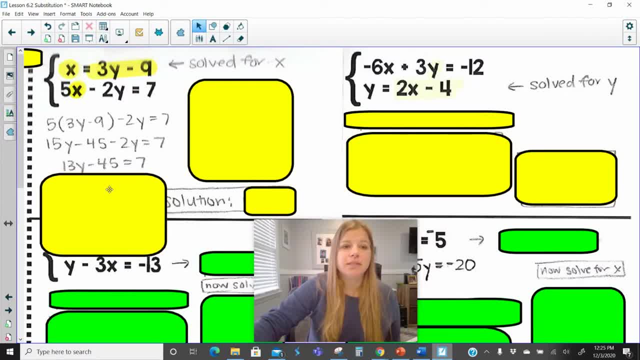 which means now, after doing some distributing, combining like terms and solving, I end up getting a value for y. But remember, in our graphing of systems of equations, video, the solution was an ordered pair. So if you have the y coordinate, well, I now need the x coordinate. 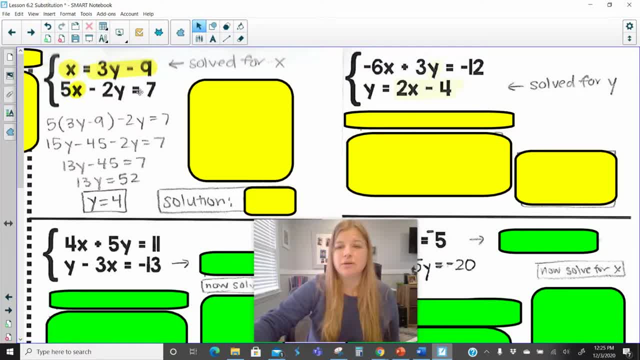 And if you need to solve for x, you could technically use either equation, But if you need to solve for x, you may as well use the equation that is already: x equals And since we now know what y is equal to, y is equal to 4,. 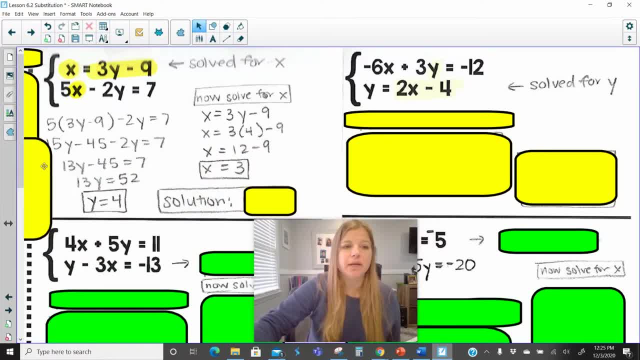 I simply plug that 4 in for y. I do my solving Now. remember the solution is an ordered pair and an ordered pair always written as the x value comma the y value. So my solution is now 3, 4.. 3, 4 is an ordered. 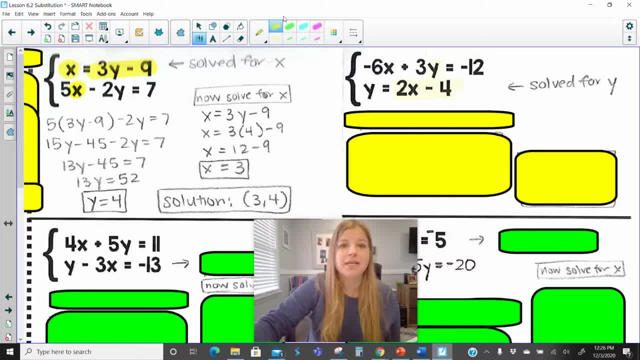 pair. that would give you a true statement for either one of these equations. So if I showed a really quick example of that and let's say I plugged in a 3 for x and a 4 for y, Let's see: 3 times 4 is 12.. 12 minus 9 is 3.. It works If I plug in a 3 and a 4 here. 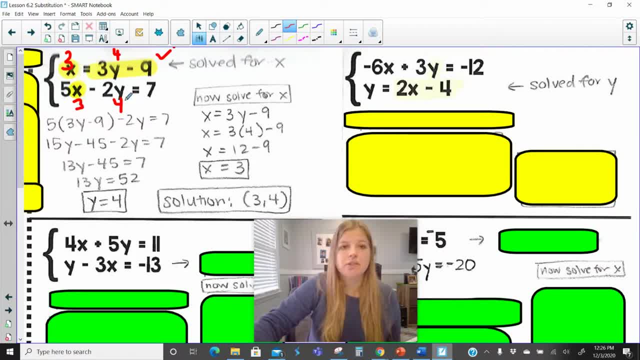 5 times 3 is 15.. 2 times 4 is 8.. 15 minus 8 is 7.. It works. Okay, let's take a look here Now. in this one, the second equation has the variable by itself. So y is equal to everything, that is 2x. 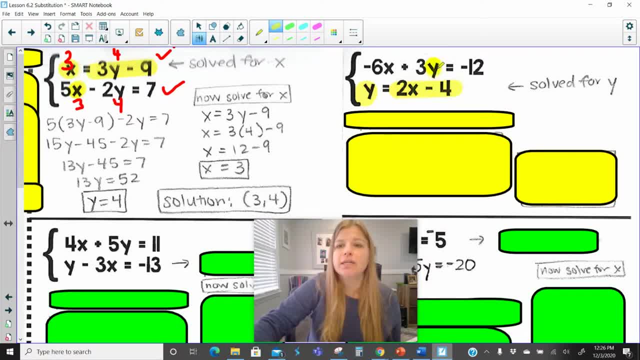 minus 4.. So that means in the first equation, wherever I see the y, I'm going to substitute in everything that y is equal to. So let's take a look In this first equation now. that would become negative 6x plus 3.. 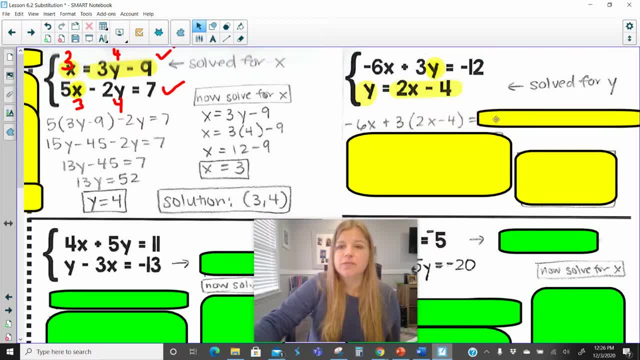 Then it's going to be open parentheses. 2x minus 4 equals negative 12.. So in this case, the variable, the equation that was already set equal to a variable, happened to be the second equation. It doesn't matter, We're going to go ahead and distribute And something we're going. 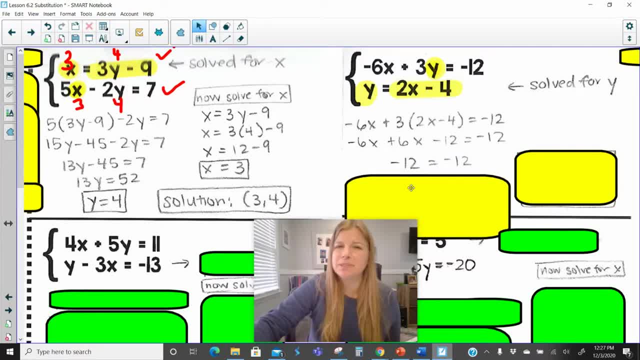 to notice. special about this equation is that my variables end up simplifying out and I'm left with negative 12 equals negative 12, which is actually a true statement. And remember what the solutions are. when you have a true statement in an equation, That's when it's 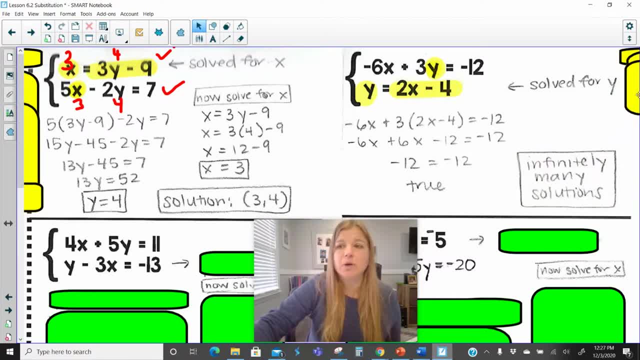 infinitely many solutions. In a basic equation it would be all real numbers, we would be able to say, But in this case it's infinitely many. So what do you think that means about the lines of these equations if I was to graph them? Well, if it's infinitely many, remember that means that 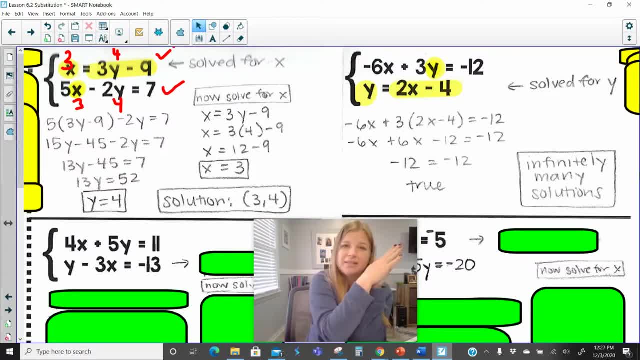 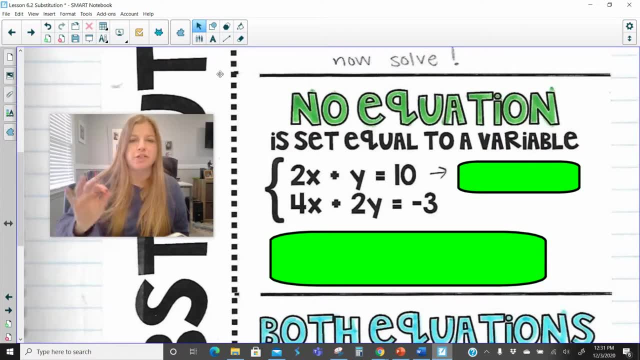 if I was to graph these two equations, they're actually going to be the exact same line. Okay, so now we're going to take a look at the second situation, where neither of the equations are actually set equal to a variable. So here you can see: both of them are in standard form. 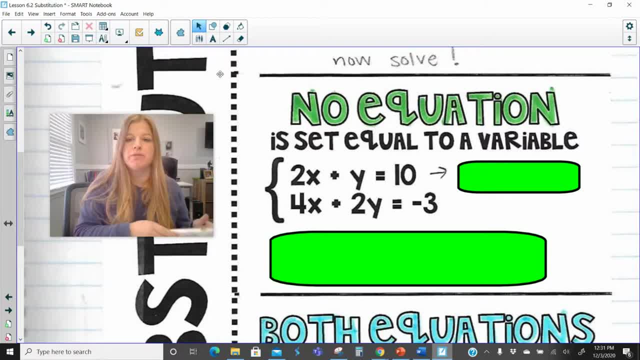 two x plus y equals 10, and four x plus two y equals negative three. And if I take a look at these two equations- two x plus y equals 10, I might say you know what? neither of them are x equals or y equals. but this first equation here might actually be really easy to get y by itself. 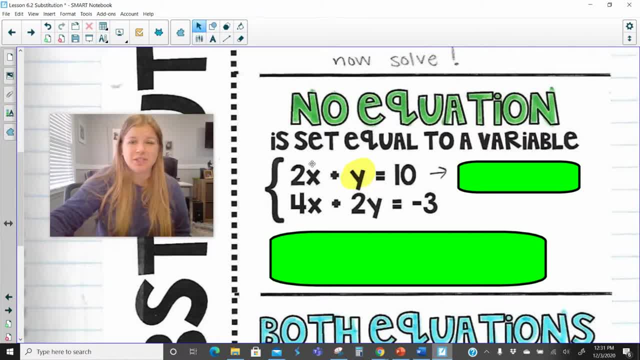 So we should notice that all we have to do to get y by itself in this first equation is subtract two x. And now, if I create that equation where it's now y is equal to negative two x plus two y, I'm going to get y by itself, And I'm going to get y by itself And I'm going to. 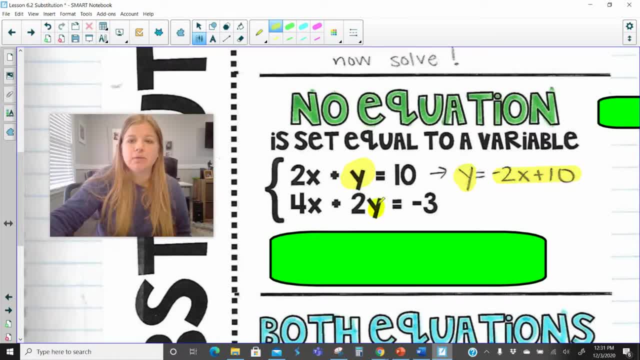 I'm able to now substitute in everything y is equal to into the other equation. So this now second equation becomes four x plus two times negative. two x plus 10 equals negative three. And I would be able to go ahead and solve like I showed you before. 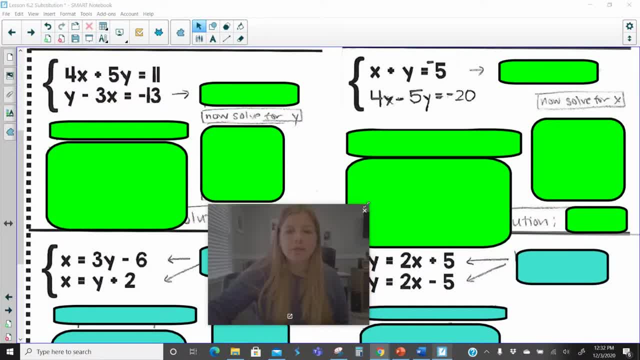 Okay, so now we are going to take a look at these two problems. Okay, so now we're going to take a look at these two problems in green. So both of these systems do not have a y equals or x equals. But if I look at this first system here, four x plus five y. 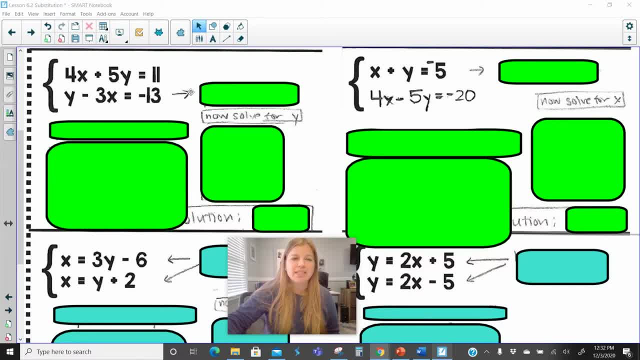 equals 11, and y minus three x equals negative 13.. I think it's going to be pretty obvious to us that this second equation is going to be really easy to get y by itself. So just by adding three x on both sides, I end up getting y equals three x minus 13.. So that means everything y is equal to. 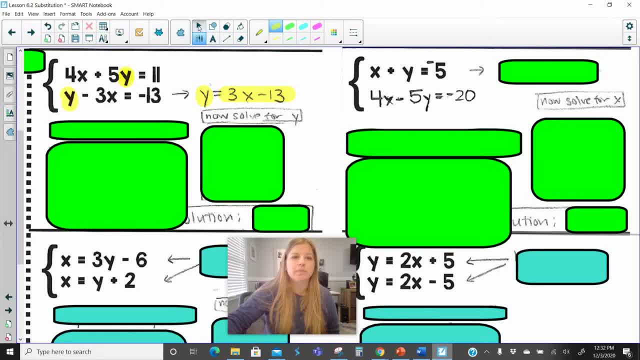 is going to get substituted in for y into the other equation. So now, instead of four x plus five, y equals 11, it will look like four x plus five times three x minus 13 equals 11.. We know the deal here. we go ahead and distribute, combine like terms, solve, and we end up getting our x. 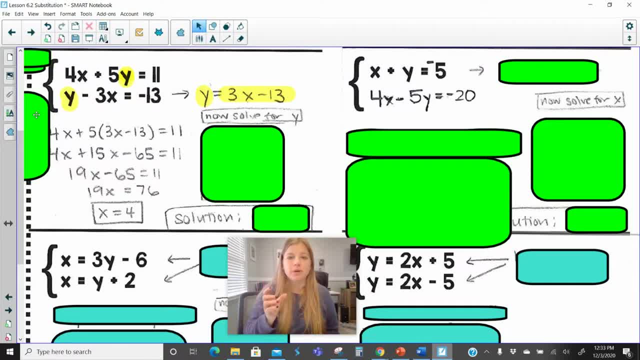 coordinate. Now we know we need a coordinate pair as a solution. So if we have our x, we now need to use the y equals equation, And the easiest way to solve for y is use the y equals equation you already have. We substitute in our x value of four and then we're able to get y is equal to. 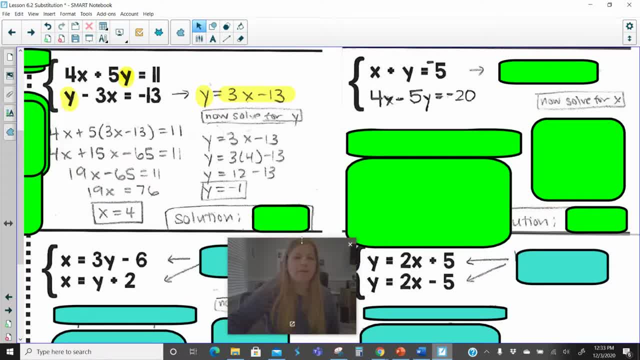 negative one, which means our solution is four negative one. Now, something else to just think about, then that would mean if I was to graph these two equations, because there is a solution that means that those lines are just simply intersecting. Next one: x plus y equals negative. 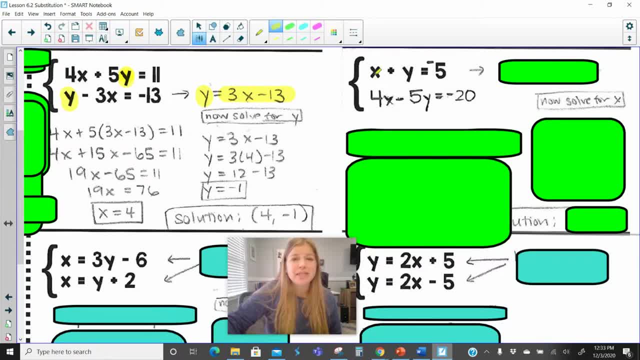 five. Now, technically we're going to be able to get y equals negative one, but we're going to. I could get x by itself really easy by subtracting y, or I can get y by itself by subtracting x rather. So either method is completely fine, And what I ended up doing here is I decided to get 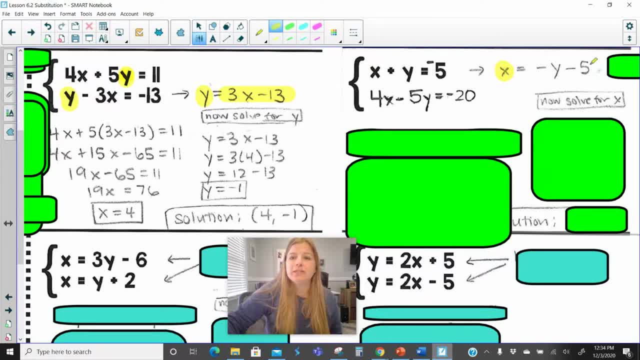 x by itself. So to get x by itself, I subtracted y on both sides. Either method will work, though, guys, I promise you. And so that means, where I see x in my other equation, I can substitute everything. x is equal to. And again, notice when you have. 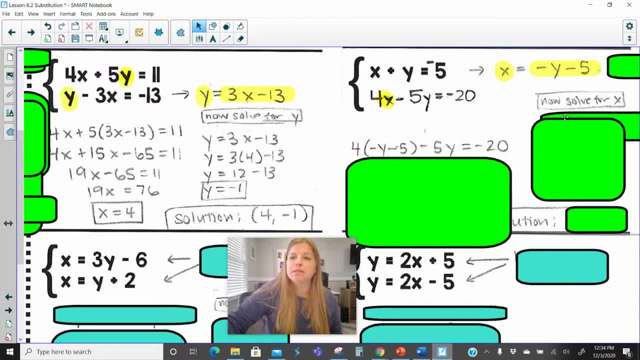 more of an expression, you need to make sure you put parentheses around that expression. Then it's business as usual. we are distributing, combining like terms solving for y. This solution of getting y equals zero is really important. It reminds us that zero. 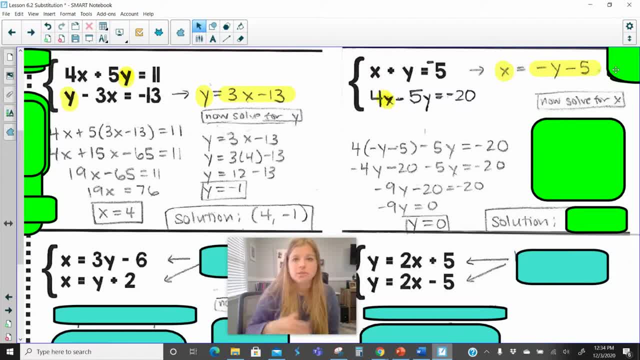 is an answer. Okay, zero doesn't mean there's no solution, you're not doing anything wrong. And then, of course, now solving for x, substituting in that zero for y, in that x equals equation, and then we end up getting negative five, And also something to keep in mind. notice your solution. 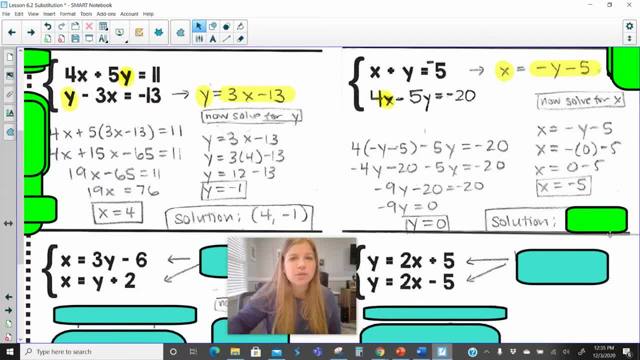 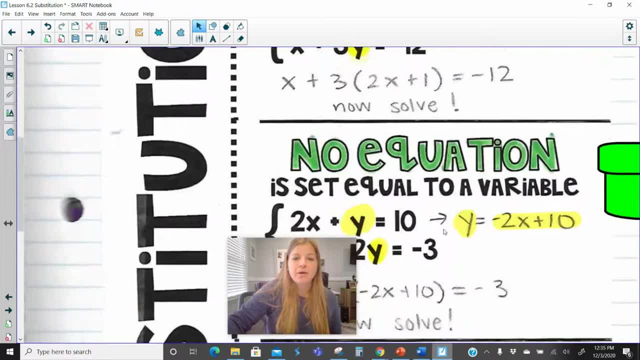 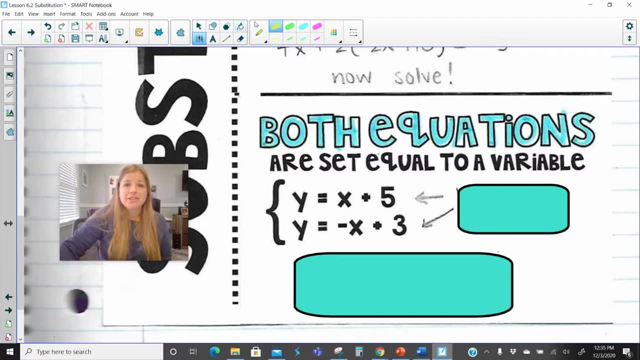 is always the x comma, the y value, not the order you solve them in, necessarily, but whatever the x value is comma, the y value. Our third case and the last case: both equations are set equal to a variable And in this case you're going to see they're. 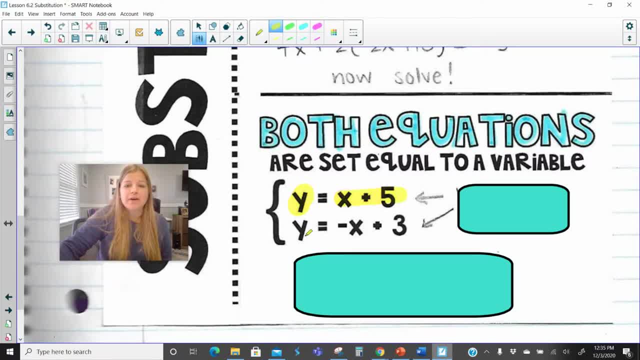 actually, both set to the same variable, y is equal to x plus five and y is equal to x minus three. That means all of those expressions I just highlighted are all equal to each other. Okay, that's. this is actually the always the easiest problem, And for some reason, 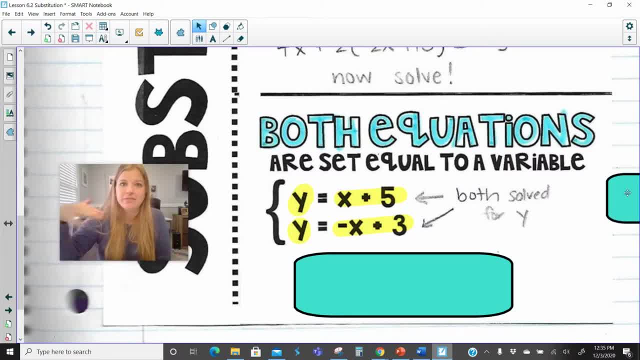 my students get tripped up on this one every single year without fail. So if y is equal to x plus five and y is also equal to negative x plus three, and think about it. what you're really doing here is you're saying all of this: x plus five gets plugged in for y into that equation.